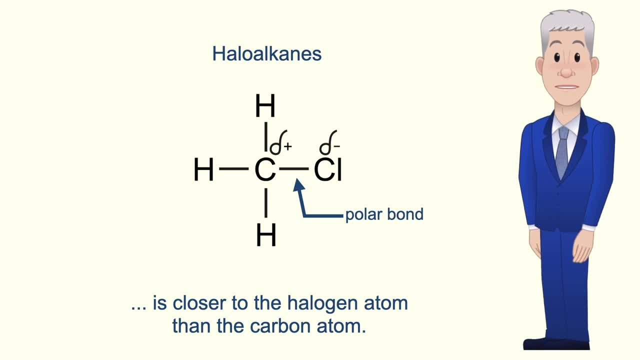 covalent bond is closer to the halogen atom than the carbon atom. This means that the halogen atom has a partial negative charge and the carbon atom has a partial positive charge. Now, this bond polarity determines how the haloalkanes react. Haloalkanes react. 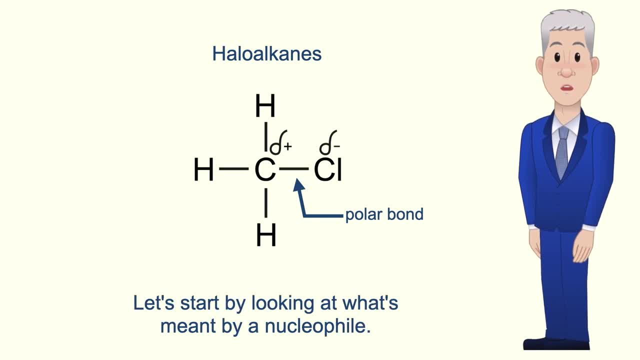 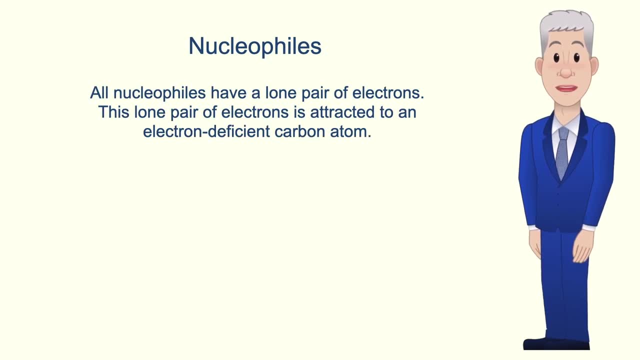 with chemicals called nucleotides. So let's start by looking at what's meant by a nucleophile. Firstly, all nucleophiles have a lone pair of electrons, and this lone pair of electrons is attracted to an electron deficient carbon atom. Electron deficient carbon atoms have a positive charge either. 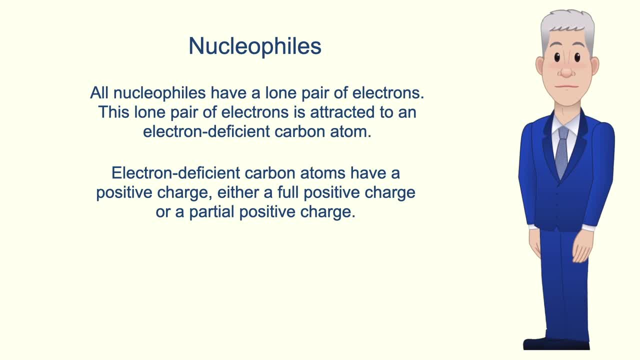 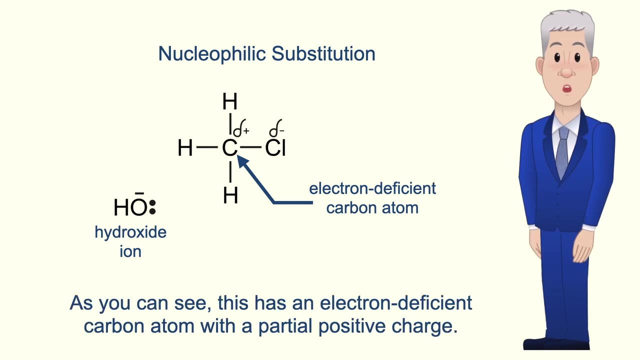 a full positive charge or a partial positive charge. The nucleophile donates the lone pair of electrons to form a covalent bond between the nucleophile and the carbon atom. OK, so let's see how this works. I'm showing you here the haloalkane chloromethane. As you can see, this has an electron deficient. 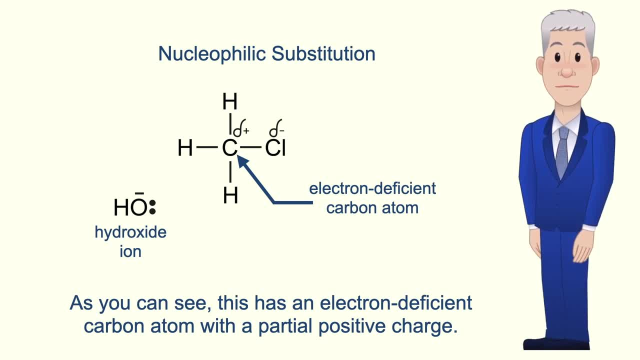 carbon atom with a partial positive charge. I'm also showing you a hydroxide ion. In the hydroxide ion, the oxygen atom has a lone pair of electrons and a negative charge, and the hydroxide ion is an example of a nucleophile. 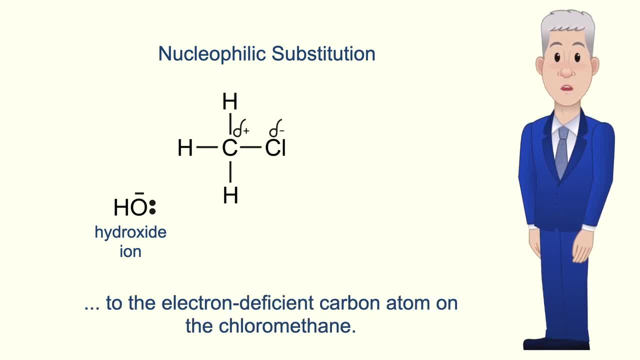 The lone pair of electrons on the hydroxide ion are attracted to the electron deficient carbon atom. on the chloromethane, The nucleophile now donates its lone pair of electrons to form a covalent bond to the electron deficient carbon atom like this: 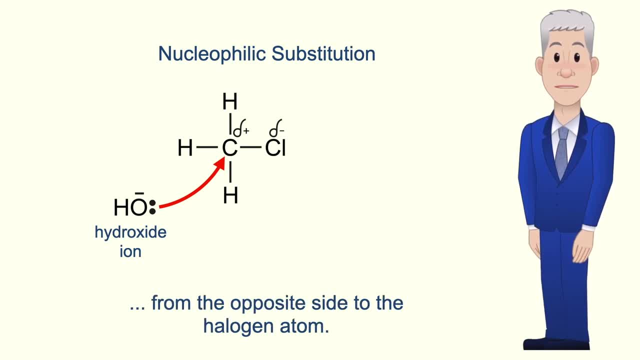 Now I've shown the hydroxide ion forming the covalent bond from the opposite side to the halogen atom. By approaching from this side, there's less repulsion between the negative hydroxide ion and the negative halogen atom. Now we represent the movement of a pair of electrons by using a curly arrow and you 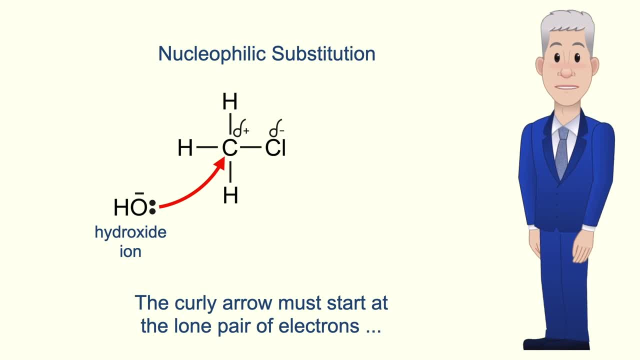 need to draw this very carefully. The curly arrow must start at the lone pair of electrons and end at the electron-deficient carbon atom. Now, a carbon atom can have a maximum of four covalent bonds, So at the same time, the covalent 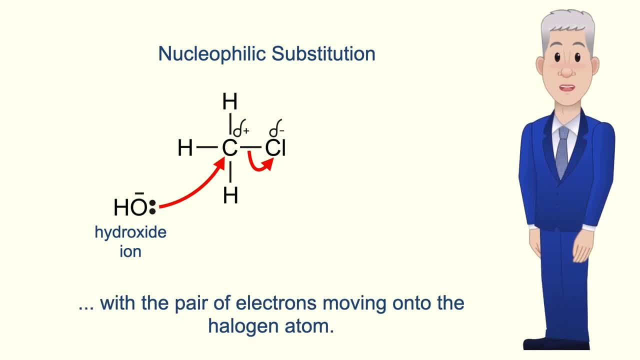 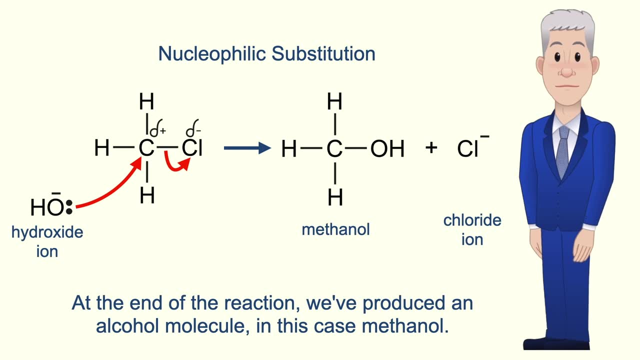 bond between the carbon atom and the halogen atom breaks, with the pair of electrons moving on to the halogen atom. This is an example of heterolytic fission. At the end of the reaction, we've produced an alcohol molecule, in this case methanol.